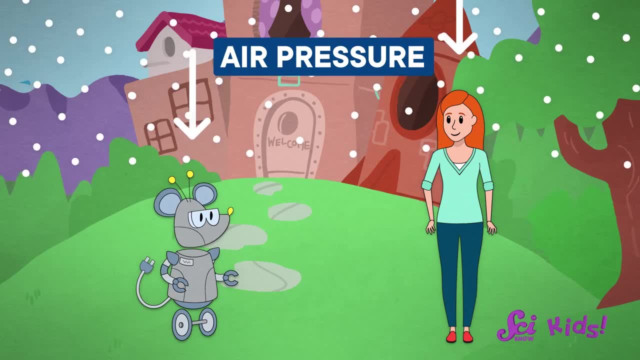 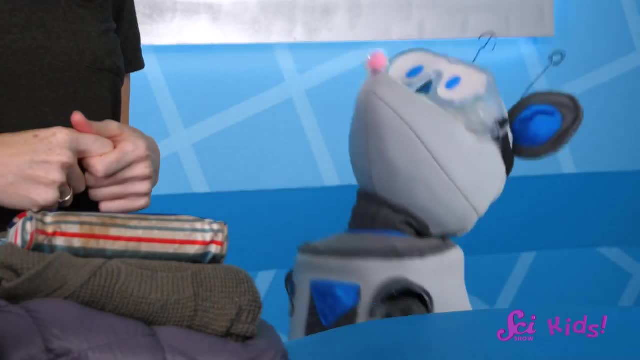 That's called air pressure. But air pressure doesn't only push on things, It pushes down. The shape of an airplane wing can make air push it up instead. Here let's check out a picture of an airplane to help show you. Here are the wings. 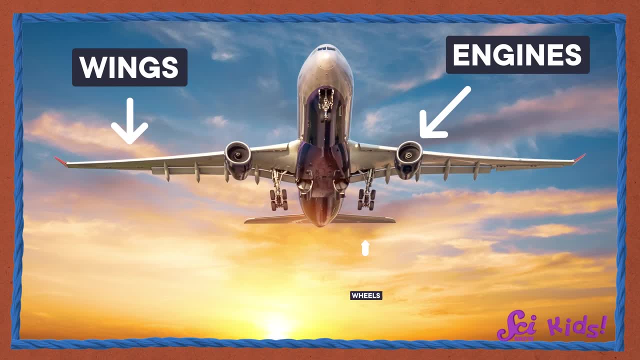 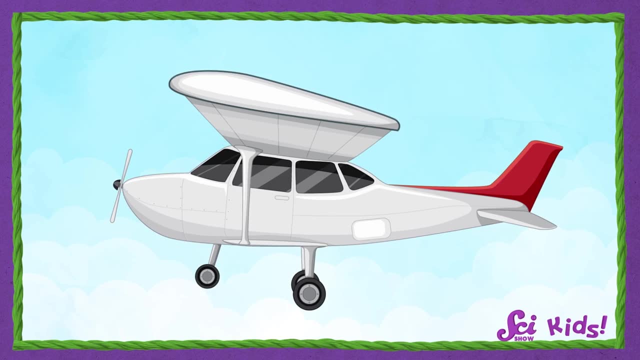 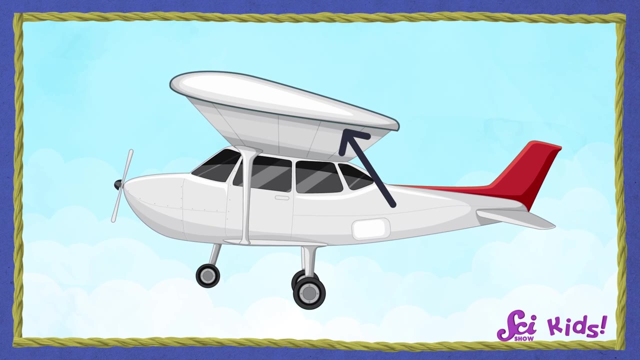 And these big round things are the engines. You can see the wheels that the plane uses on the ground too. But let's look at the wings of this airplane. What do you notice about their shape? Oh yes, great observation. This airplane's wings are kind of flat on the underside, but the top is a little bit rounded and curved. 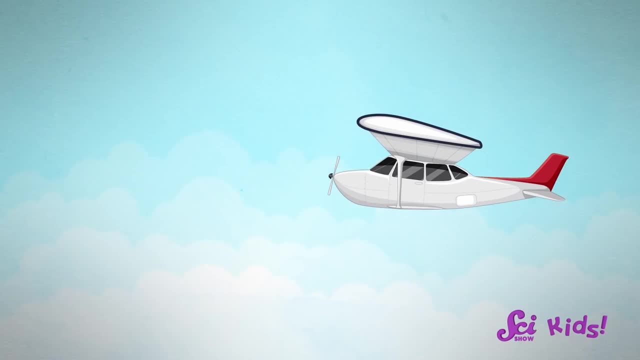 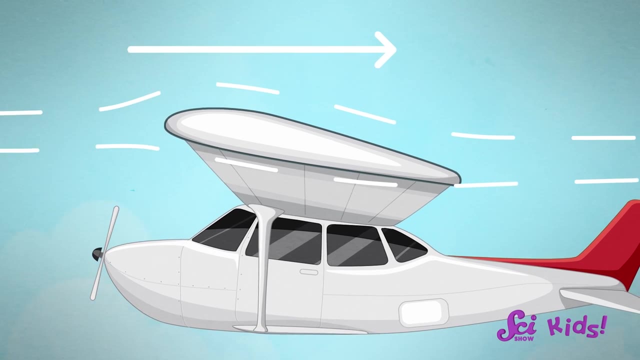 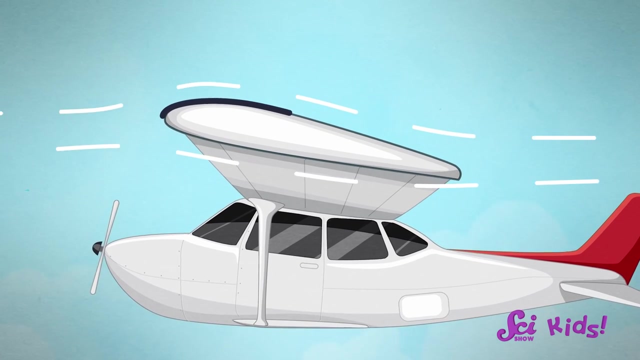 Because of an airplane wing's unique shape, air moves differently above and below it as the airplane moves forward. from thrust, The air has to move from the front of the wing to the back as the airplane moves forward. But in order to get over the rounded top edge of the wings, the air has to move faster than it does to go underneath the flat bottom of the wing. 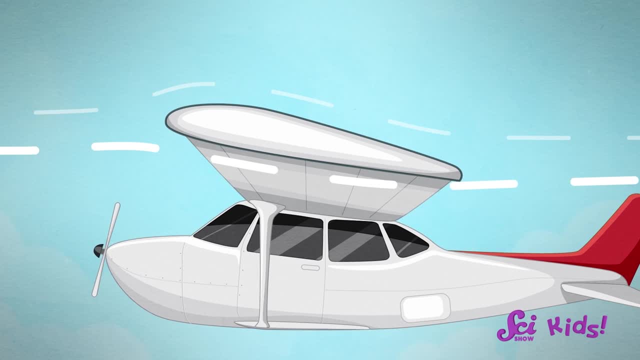 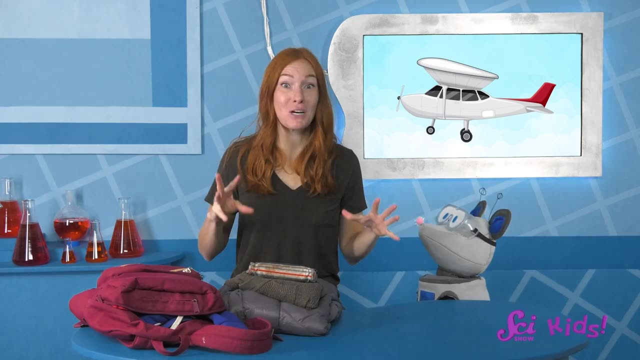 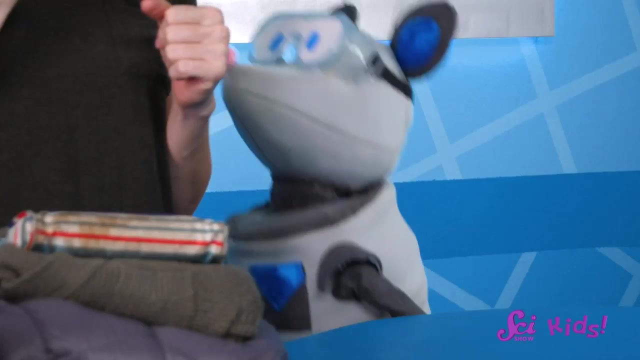 Because the air underneath the wing isn't having to go as fast, it is able to put more of a push on the wings than the air above the wing. This pressure pushes on the airplane wings And it pushes more up from the bottom, making the plane go. You're right Up. The push from the slower air under the wings is another force called lift. Lift does exactly what it sounds like: It lifts the airplane wings up, Up into the air, bringing the whole airplane up, up, up. 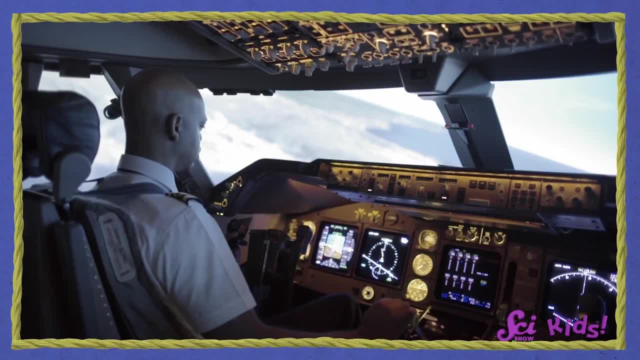 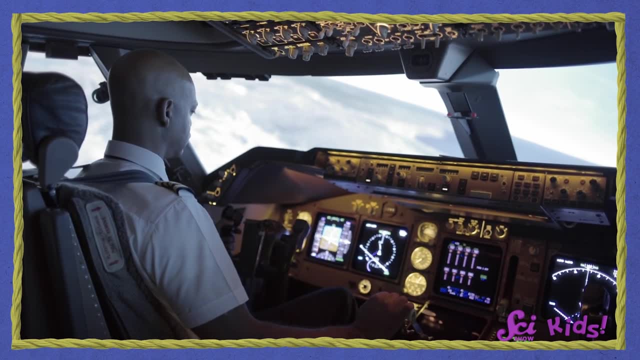 The airplane won't be lifted up forever. Squeaks. Pilots control how high up the airplane is lifted and whether it turns left, right or back down toward the ground using the engines and special panels on the wings and tail of the airplane. 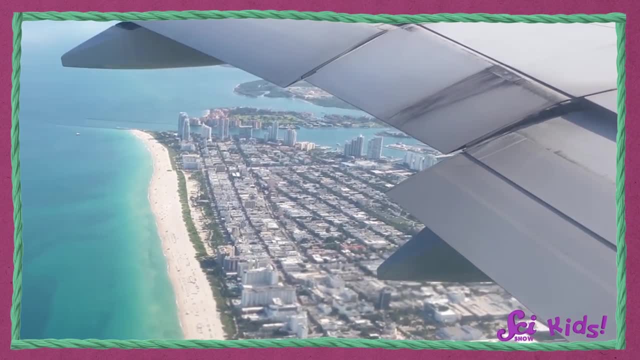 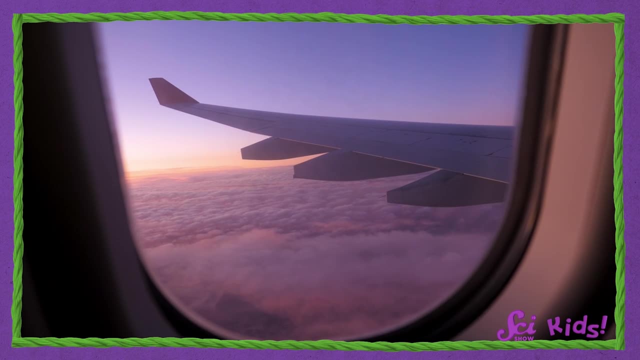 Those panels can change the way air moves around the wings, So they change the way it pushes on them too. Depending on where you sit in the airplane, you might even be able to see some of these special wing panels move as we take off and fly. 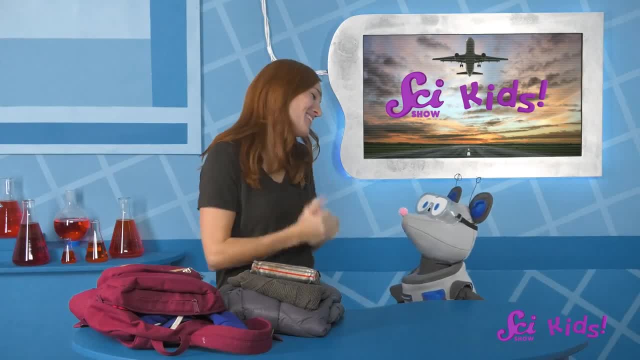 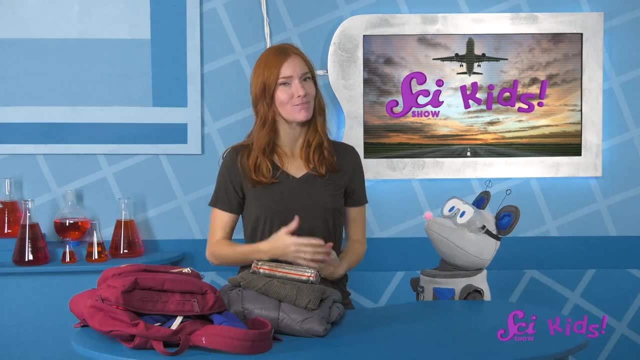 Oh, I'm so glad that you're excited to watch the airplane work Squeaks And I'm glad that this is making you feel better about your first airplane ride. You know, sometimes just understanding something can make it a lot less scary.